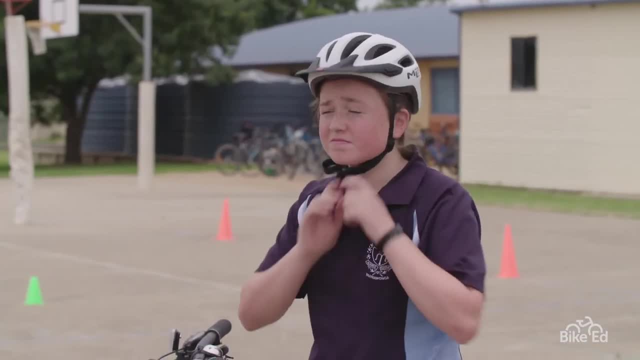 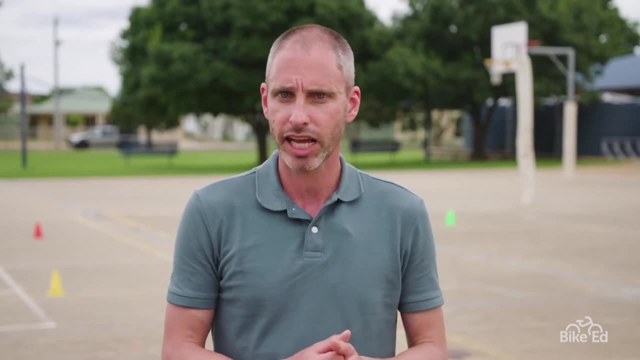 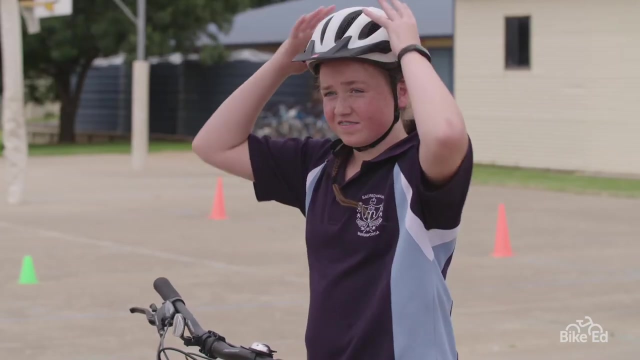 right size and be worn correctly, otherwise it won't work. The helmet should sit about two fingers above your eyebrow. The straps on each side should be adjusted to meet just under your ear. The chin strap should fit snugly. Make sure that the helmet fits snugly on your head. It needs to be the right size or it. 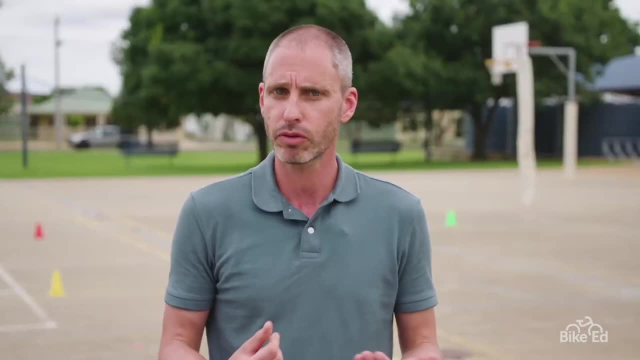 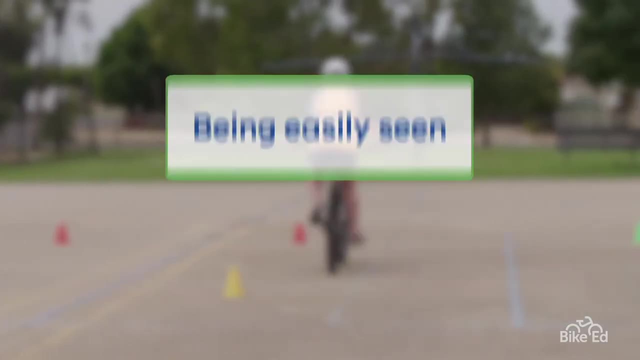 won't protect you in a crash. If it's too big, it would shift around on your head. If it's too small, it won't sit fully on your head. It's essential that other people using the paths or road can easily see you. The 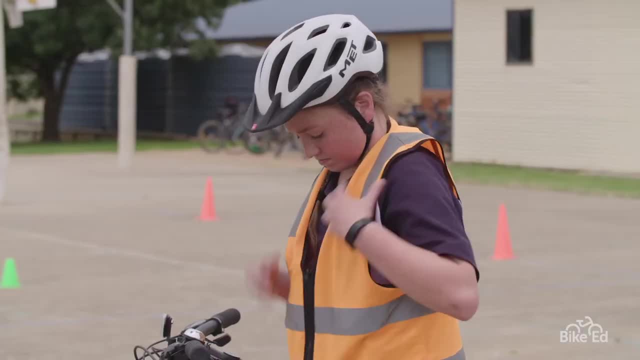 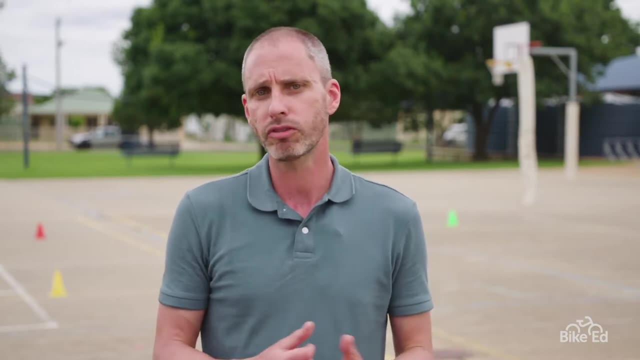 best way to do this is to always wear bright coloured clothing when you ride. If you're riding when the light conditions are not good, such as early morning or late afternoon, or when it's foggy, then you need to use lights on the. 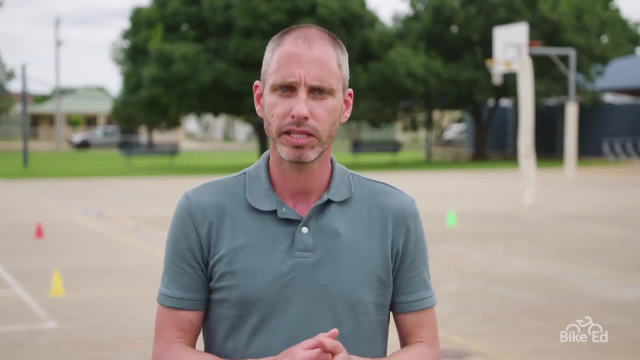 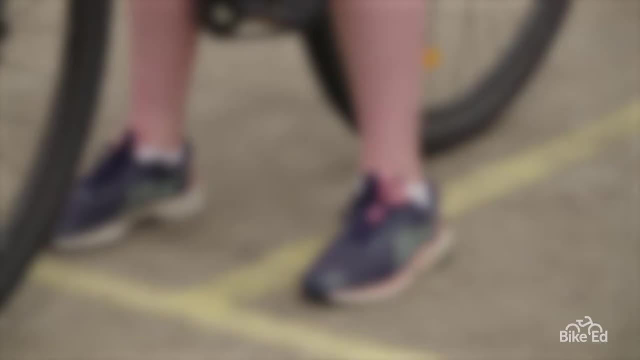 front and rear of your bike. Remember you need to be seen. to be safe, It's important that you wear non-slip closed-toe shoes. This is to protect your feet and also so you don't slip on the pedals or ground when you stop. 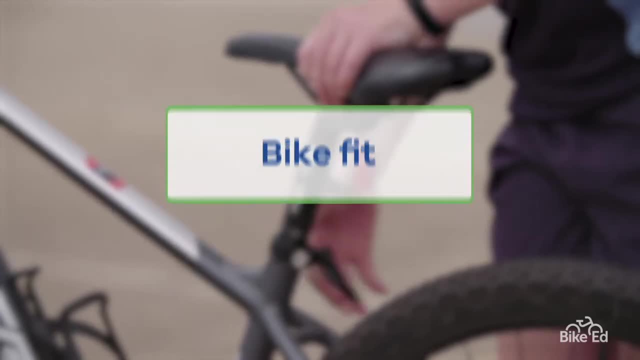 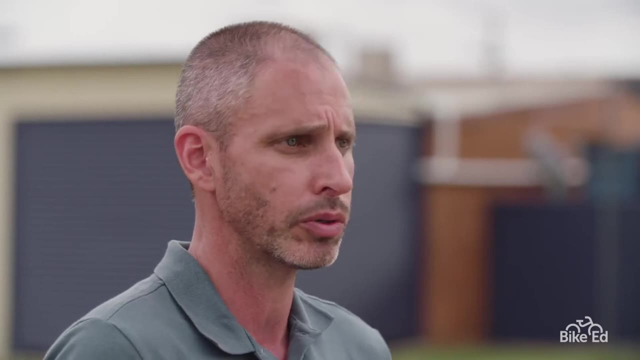 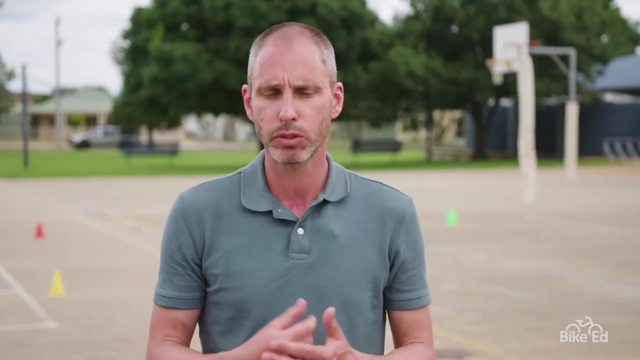 It's important that your bike fits you correctly. It means that you have the right size bike and it's adjusted to suit you. The frame of the bike needs to be the right size. Ideally, you should have a 5 to 10 centimetre gap between your crotch and the top tube when 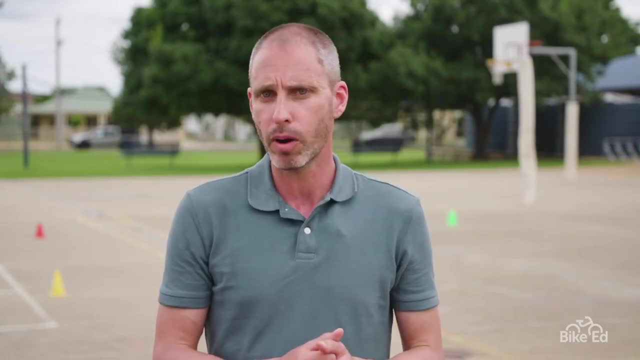 you stand over the bike. This will be a smaller gap on a road bike, about 3 centimetres. Thank you. If it's more than this gap, the bike frame is too small for you, and if it's less or there's no gap, the bike frame is too big for you. The seat should be. 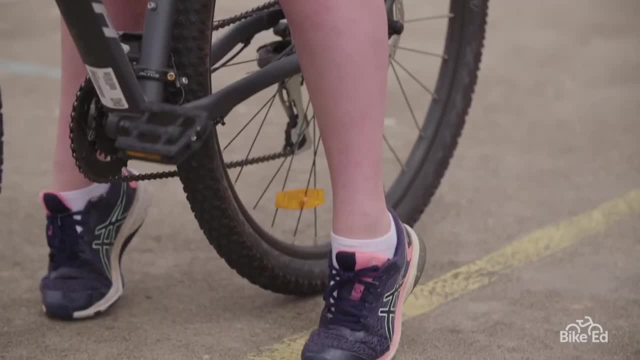 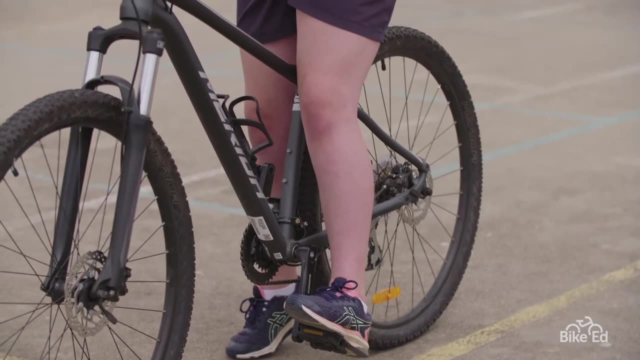 adjusted so that when you're sitting on the bike, you can just touch the ground on your tippy toes. Another way to check the seat height is to put your heel on the pedal and check whether your leg is straight when the pedal is at its lowest. 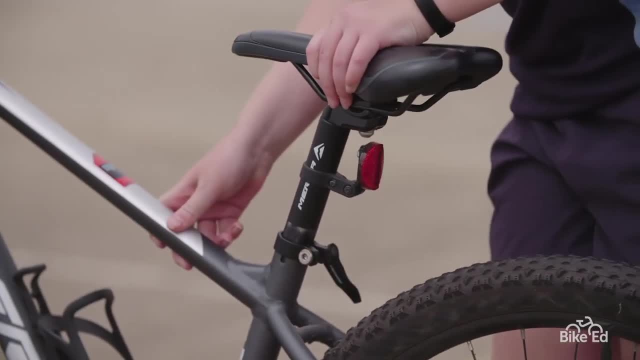 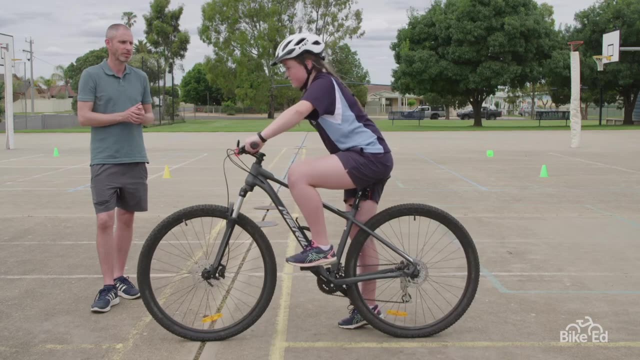 position. You can easily adjust your seat height if you need to When you're sitting on the bike. as a general rule, you should be leaning slightly forward when gripping the handlebars. You can check this gap between the bike seat and the handlebars.